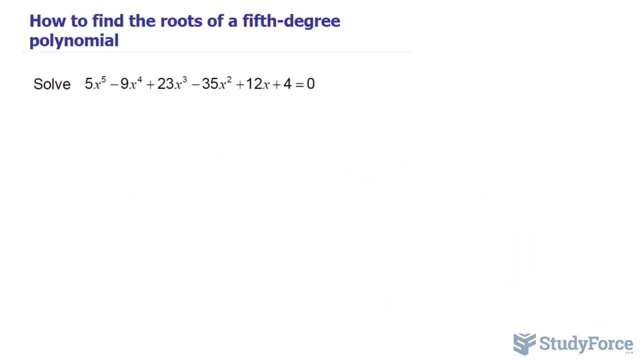 In this tutorial, I'll show you how to find the roots of a fifth degree polynomial. The equation that we're working with is shown right here and, as you can see, the highest degree is five. If you've watched my previous video on solving a quartic, you'll find that 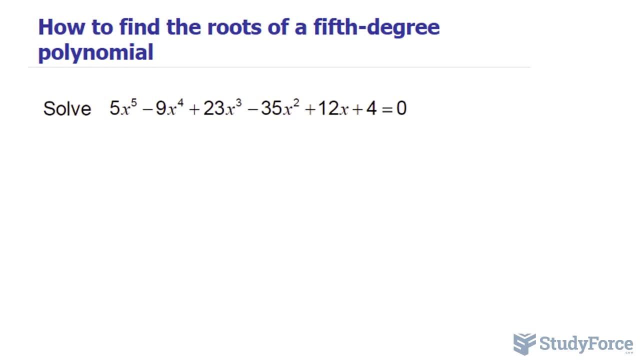 this one's a little more involved. Just like before, I'll be using the rational zero theorem to help me throughout the process. The rational zero theorem is a way to find a potential list of roots. given what we know about the leading coefficient and the constant, I'll 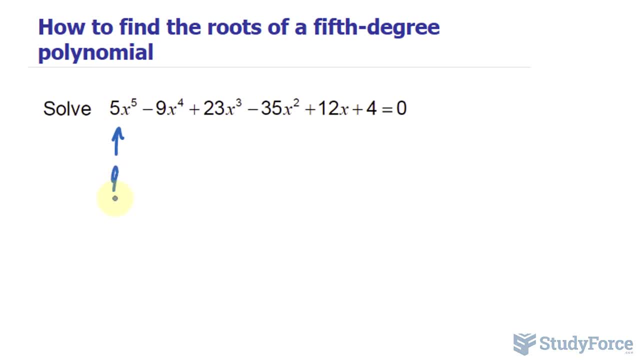 call the leading coefficient q, so we'll call five q and four will be p. According to the rational zero theorem, if we divide factors of p with factors of q, that will generate a list of potential roots. Now, none of those roots that we generate will guarantee an actual 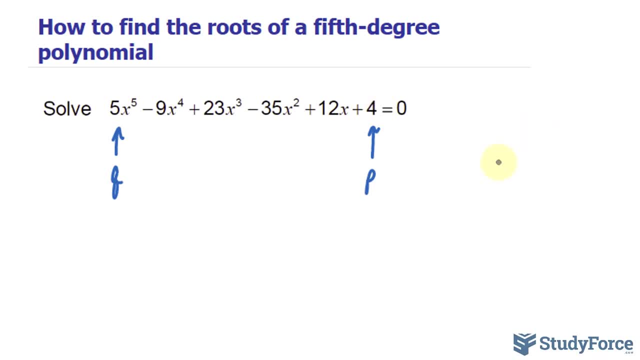 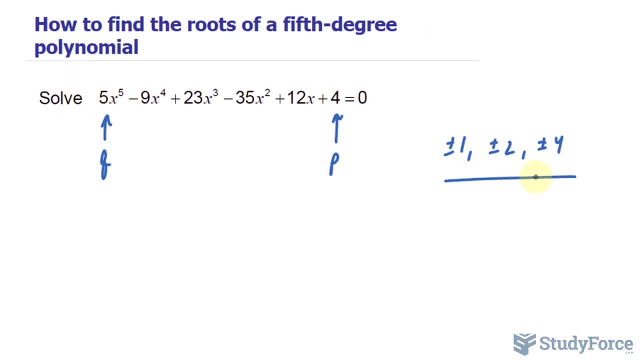 zero, but it helps us narrow it down. So factors of four include plus minus one, plus minus two and plus minus four. Factors of five: well, it's a prime number, so it's plus minus one and plus minus five. 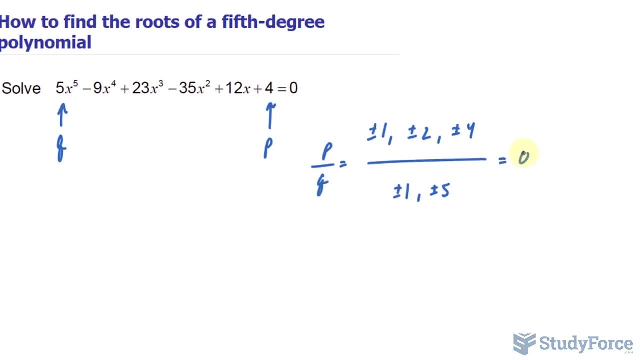 So, as you can see, I'm dividing p's with q and I end up with quotients. Remember, quotients are numbers from division statements, answers to division statements. Let's find out what they are. We have one divided by one that's plus minus one that's plus minus one over. 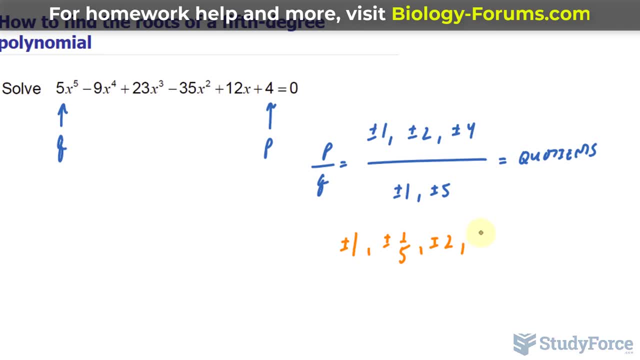 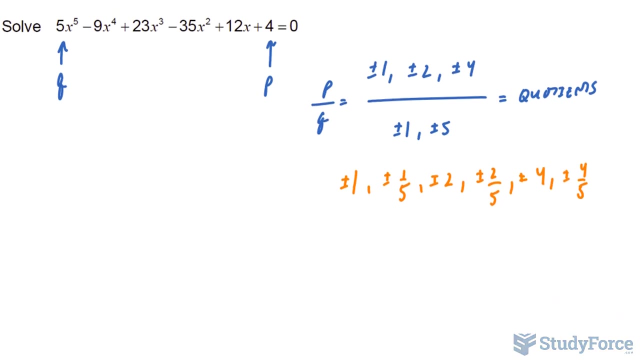 five. Now we do the twos plus minus two plus minus two over five, And the four, that's fours, are plus minus four and plus minus four over five. So these are potential roots for this fifth degree polynomial And according to the rational zero theorem we have to test. 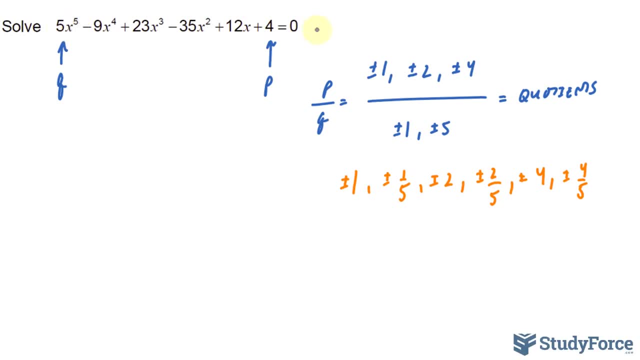 each of these quotients into the equation to see if any of them result in an output of zero. As you can tell, that would take a long time. To substitute these into the equation would take a while, So I've done it for you already and I found that that 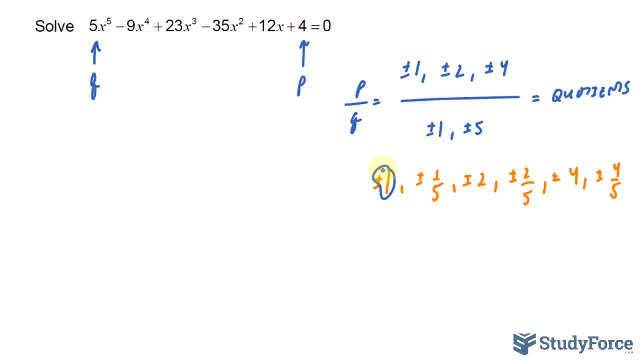 plus one is the only one out of all these that makes the quotient zero, So I'm going to use the equation equal to zero. The reason why that's important is because now we can rewrite our equation in factored form, using this as one of our factors. So I'll write: 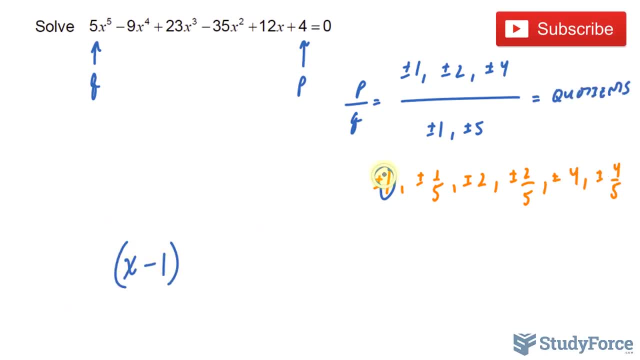 down x minus one. Notice that plus one became minus one. That's because if I were to solve the equation I would end up with: x is equal to one, So make sure you use the opposite sign when writing it in factored form. And the rest of the polynomial well to find. 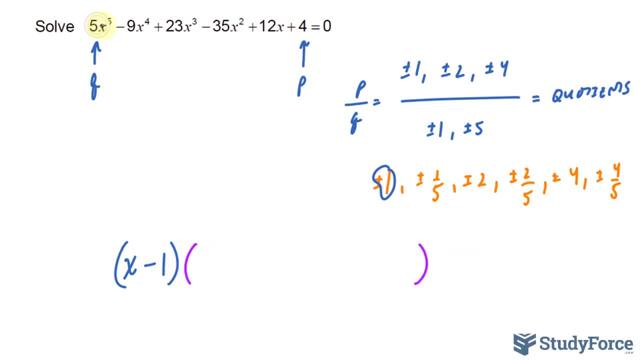 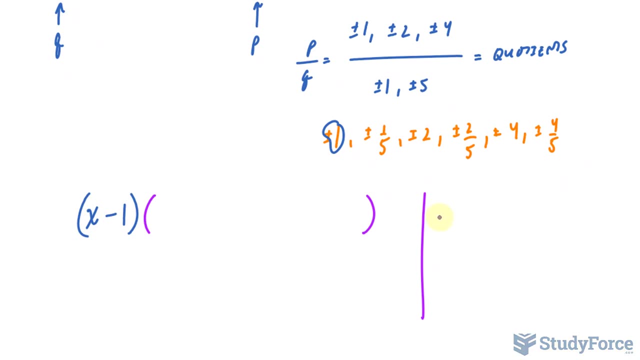 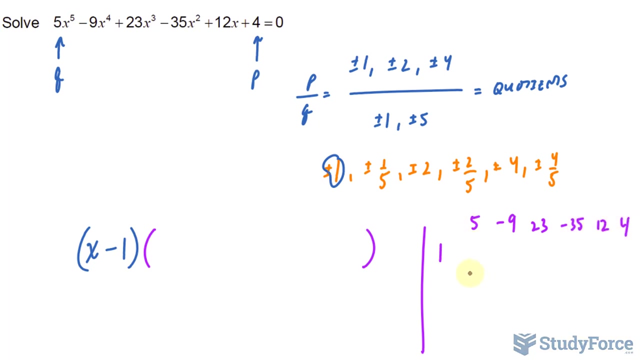 the rest of the polynomial. we have to synthetically divide this, This and one. So I have over here a synthetic division. will be positive, one with the coefficients five, negative, nine, twenty-three minus thirty-five, twelve and four. So we start by placing the 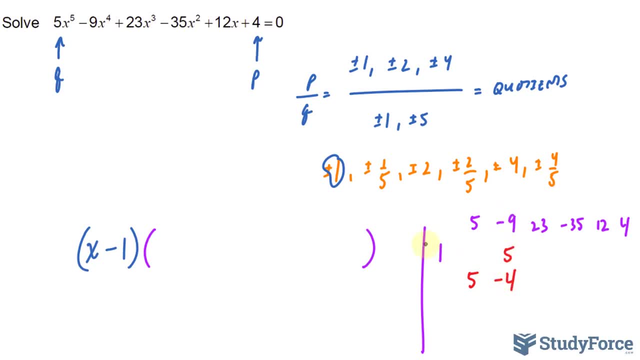 five here One times five is five Combining those. that's negative. four One times negative. four is negative four Combining those. that's ninety One times nineteen. Placing that right there, that's negative. sixteen One times negative. 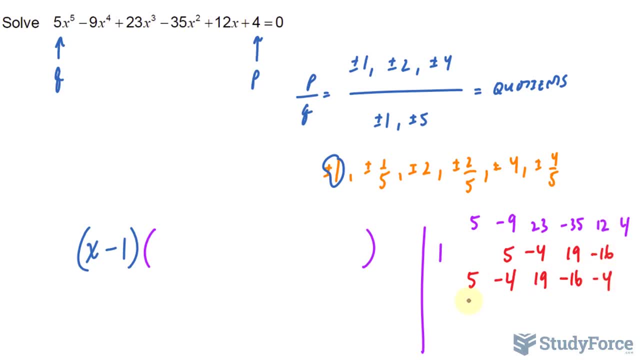 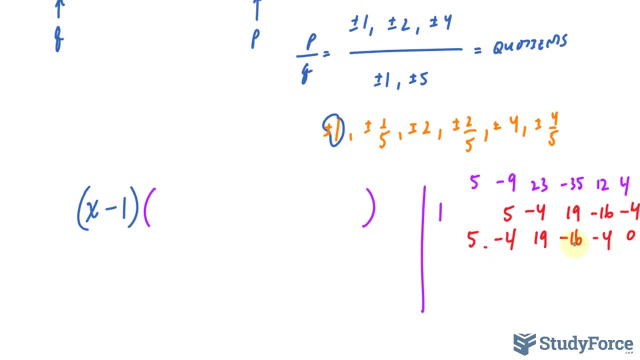 sixteen, of course, is negative sixteen. That becomes a negative four, And over here we have negative four and that's zero. So these numbers will represent the coefficient of the polynomial that's generated, which is a fourth degree, Five x to the power of four. 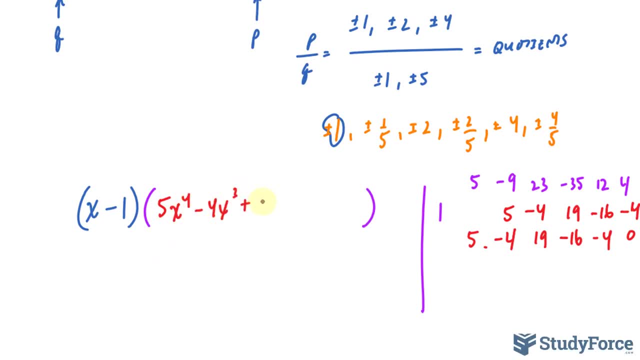 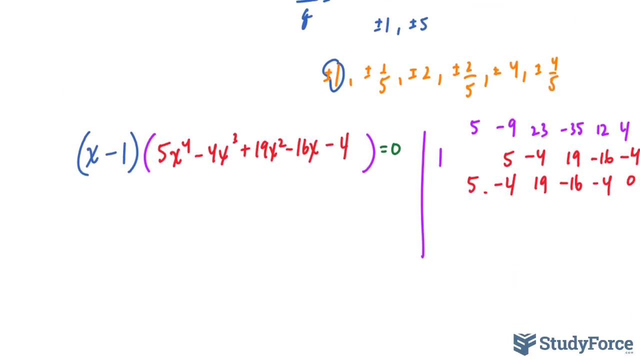 minus four, x to the power of three plus one, Nineteen x to the power of two minus sixteen, x minus four. So this is our brand new equation. It represents the same thing as this And we have to perform the rational zero theorem. 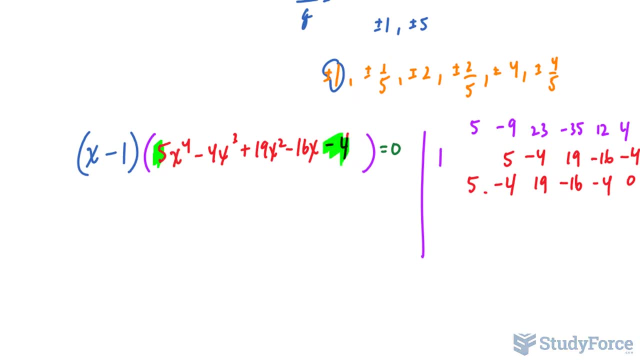 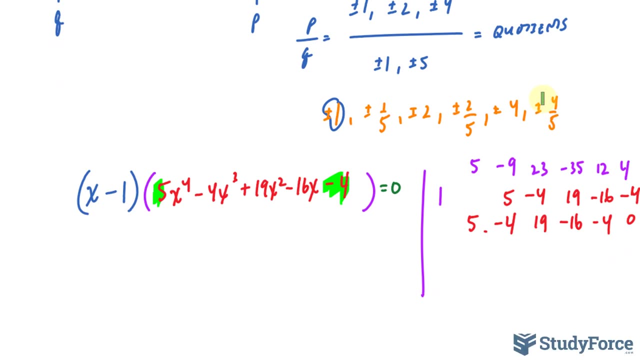 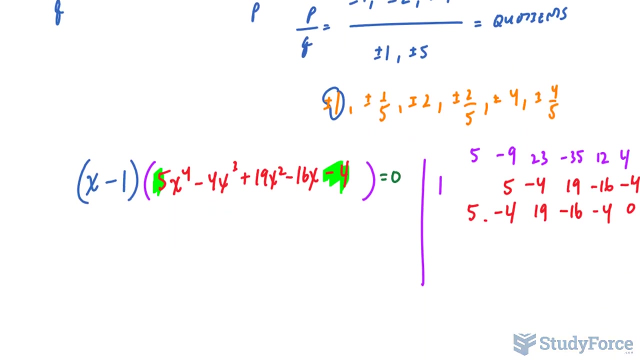 again, using five and negative four this time. Notice the difference. However, you will still generate the same quotients if you divide p and q, If you have negative four and five, as you did with four and positive five. So we'll use these again and you'll find out that if you substitute these values in 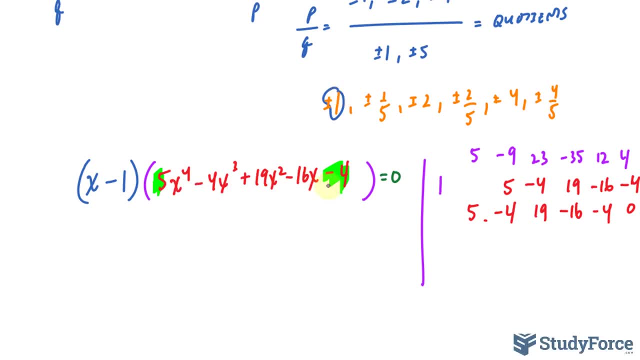 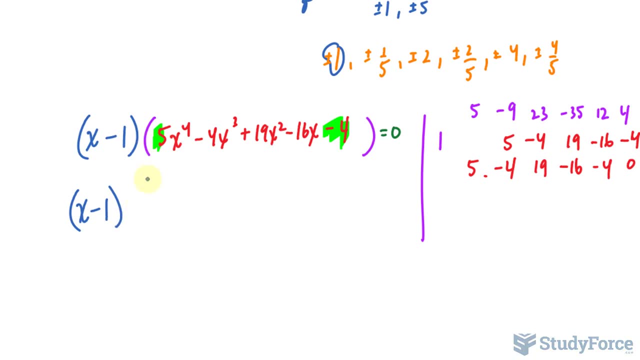 positive, one will make this into zero again. With that being said, we have to synthetically divide. I mean, we can rewrite this as x minus one, that remains the same, And then x minus one again, and now our new polynomial that remains can be found using synthetic division. 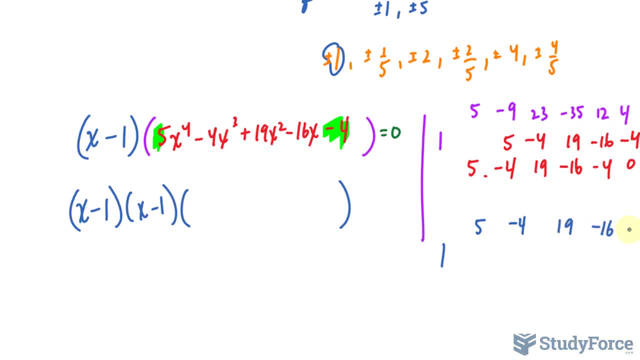 One, five negative, four, nineteen negative, sixteen and negative: 4.. Rewrite 5.. 1 times 5 is 5.. Combine those, it's 1.. 1 times 1, combine those, it's 20.. Those two make positive 4, and these two make 0. So we have 5x to the. 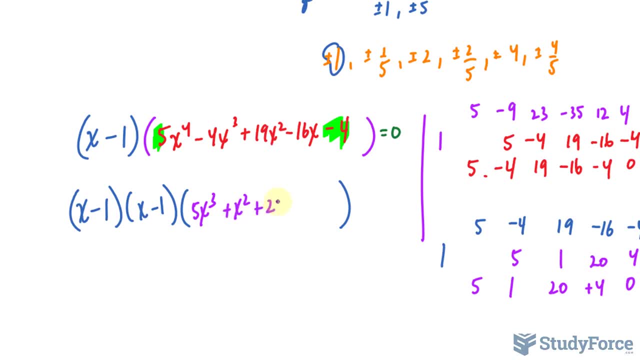 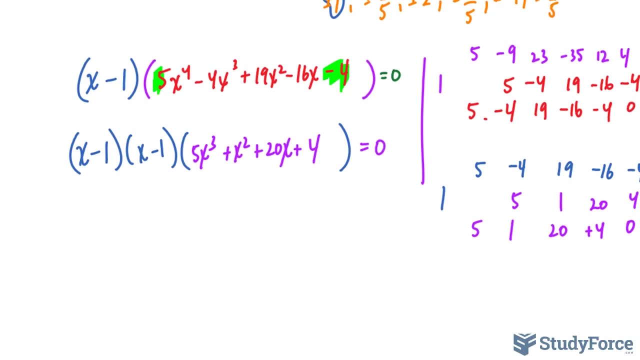 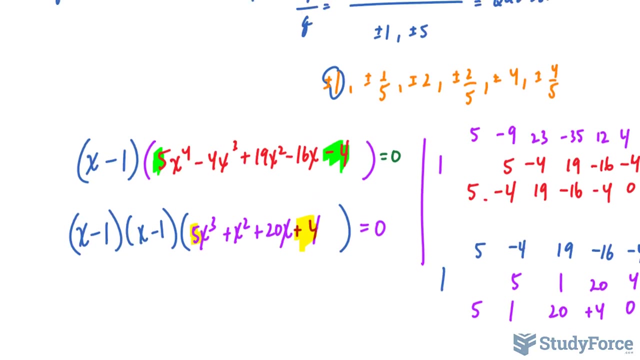 power of 3 plus x to the power of 2 plus 20x plus 4, and that is equal to 0.. We use the rational zero theorem, again with 5 and positive 4.. As you can see, they're the same as before. These will be the quotients, and this time 1 does not work. 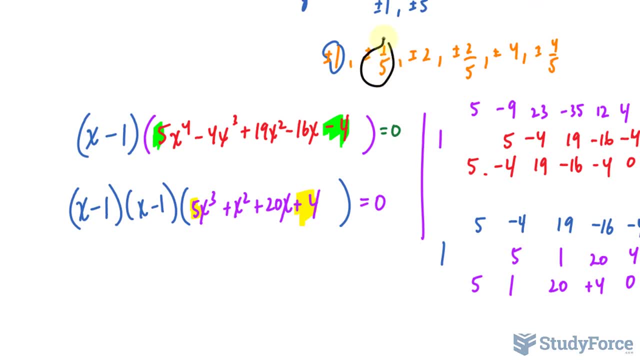 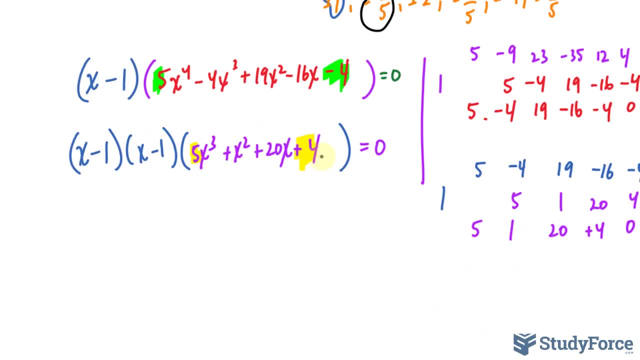 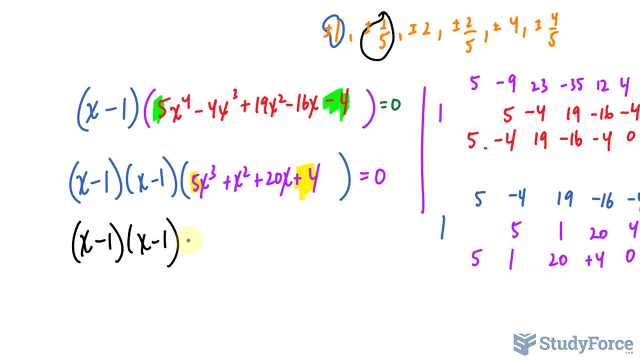 Instead negative 1 over 5 works. So substituting negative 1 over 5 into here makes it 0.. Let's use synthetic division again to break this down, But first in factored form: x minus 1, and we said negative 1 over 5, so I'll write that. 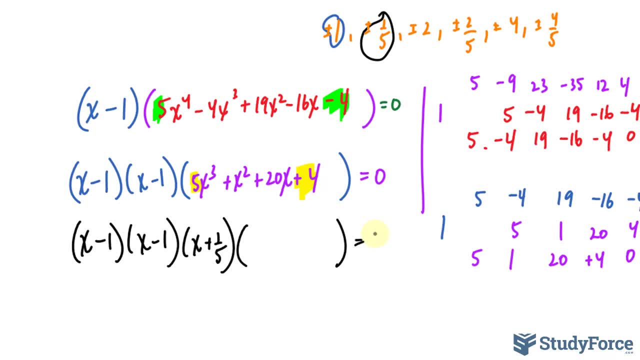 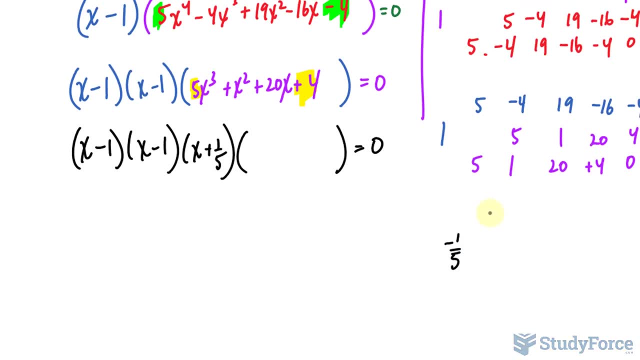 as an x plus 1 over 5.. Now the quadratic that forms will be found using synthetic division. I have negative 1 over 5.. 5,, 1,, 20, and 4.. Write down 5 here, multiply. 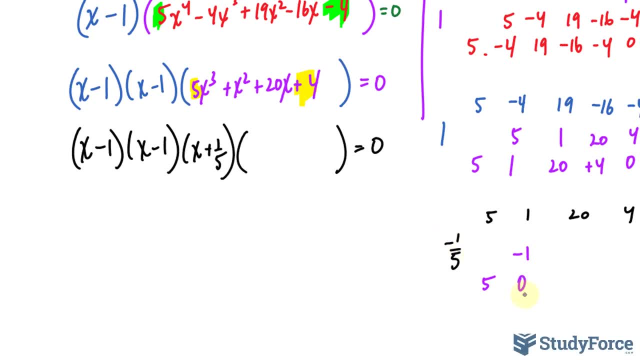 these out: I get negative 1. Combine, I get 0. This times 0 makes 0, that's 20.. 20 times negative. 1 over 5 is negative 4, and we get 5x squared. 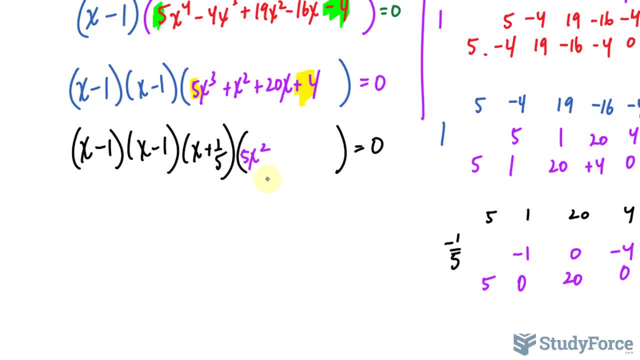 That's a 0, so we won't have an x term plus 20.. I'll factor out a 5 from here. I get 5x squared plus 4, and I'll bring that 5 over here. Now I have to solve for my x's. 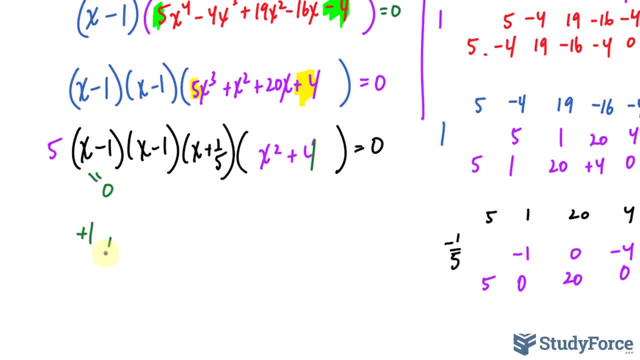 If I set this equal to 0,, I get positive 1.. Set this equal to 0, I get positive 1.. Notice that this has a multiplicity of 2,, which means that it will only touch the x-axis and not.